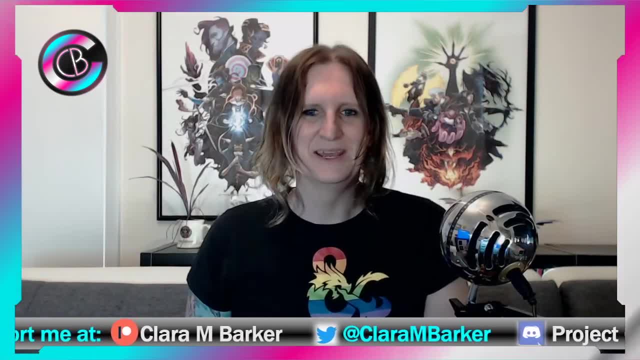 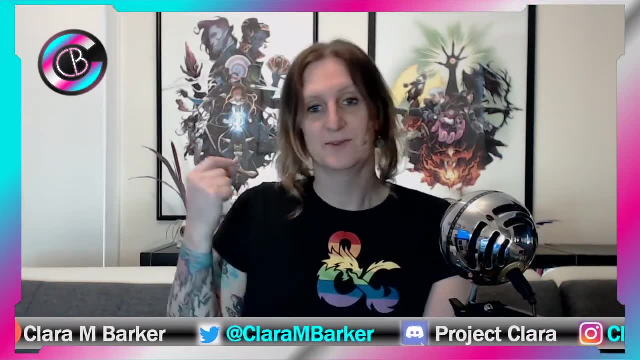 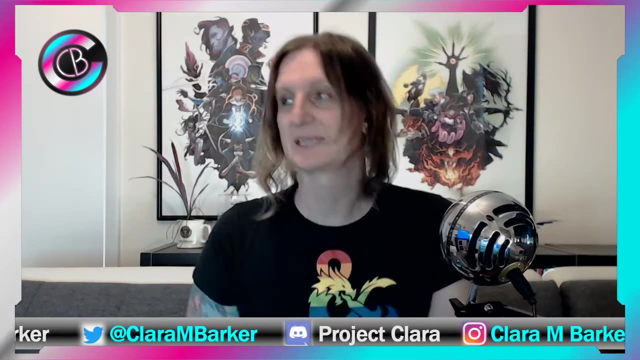 Hi everyone, how you doing? It's me, it's Clara Barker, and I'm doing another one of my science videos And the video today I am continuing my talk on superconductivity. Like I say, I'm the manager in the Centre for Applied Superconductivity in the Materials Department of Oxford University. 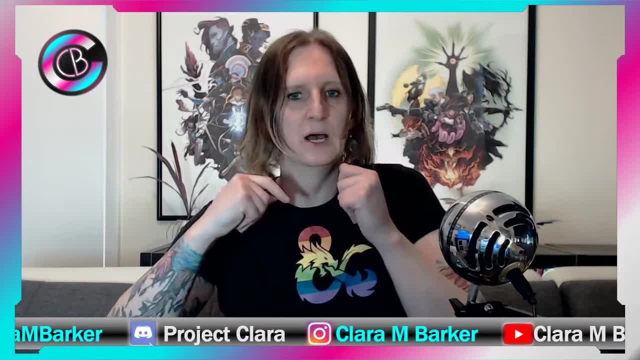 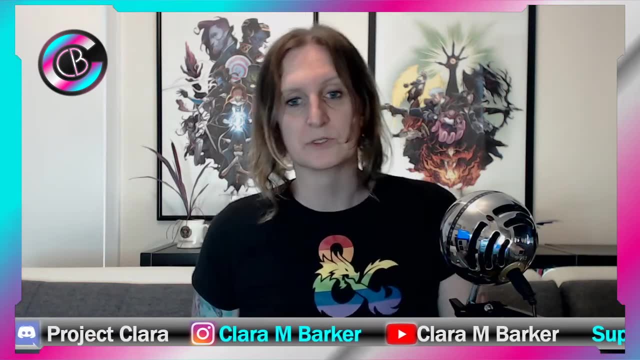 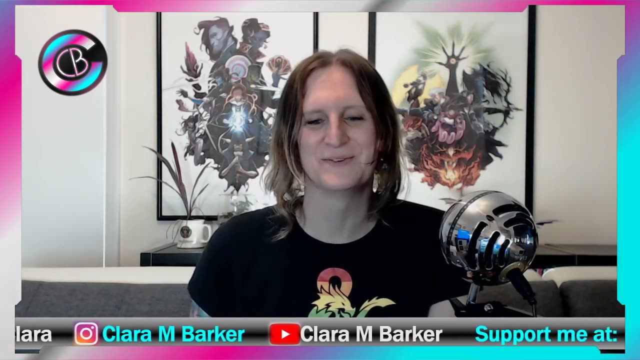 And so here I'm going over some of the basics of what superconductors are and how that happens, how it works, and just generally, hopefully some cool stuff. And I've actually got some cool little videos that I can show you today of some of the properties that I'll be talking about. 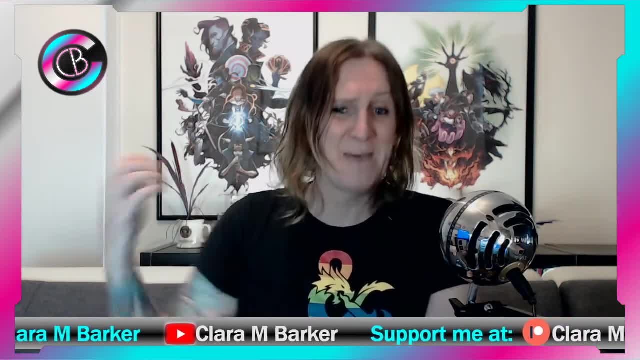 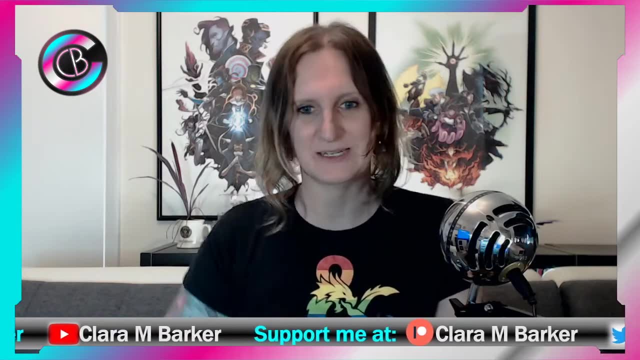 Of course I would love to be able to film them better, but I haven't been able to go in my lab for about two months now and I'm not sure when that's going to change thanks to the current coronavirus lockdown that we've got going on. So, anyway, that's done. 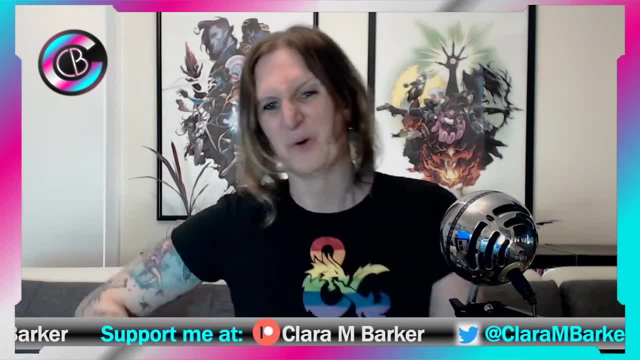 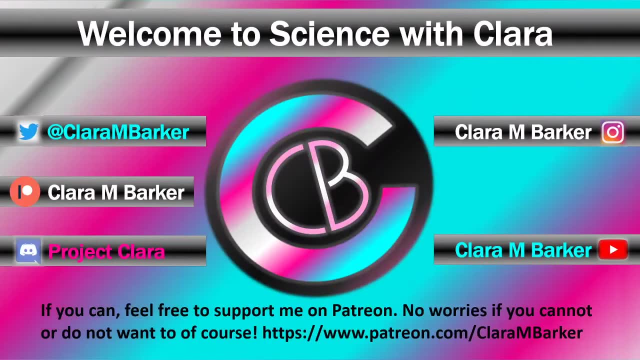 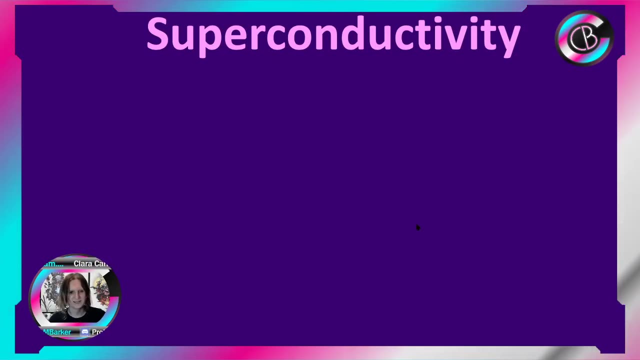 I've got some videos there and I think they're kind of cool. So, yeah, let's move on to it. Alrighty, so I've got my slide up and, like I say, I'm going to continue my talk on superconductivity. 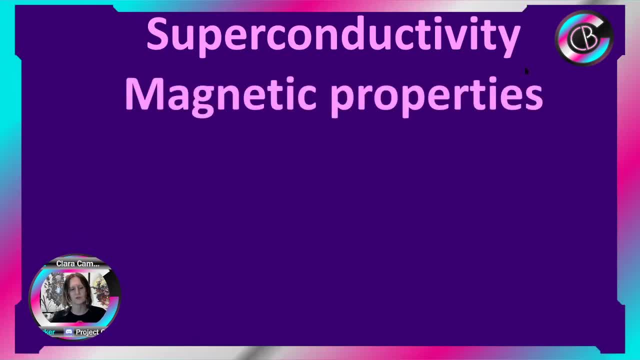 But today what I'm talking about is the magnetic properties. So these are how superconductors interact with magnetic fields. I'm talking about, say, a permanent magnet or whatever I'm going to talk. there'll be another talk where we can talk about how we can use their. 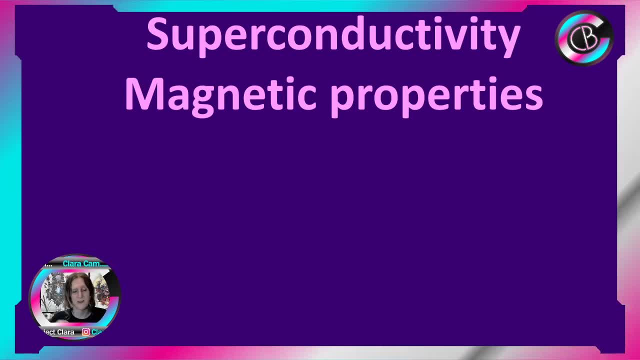 interaction with magnetic fields. but here I'm going to talk about how they interact with magnetic fields. This isn't necessarily any magnetic force that they're generating. Again, that will be in another talk. So here we're talking about the superconducting properties. 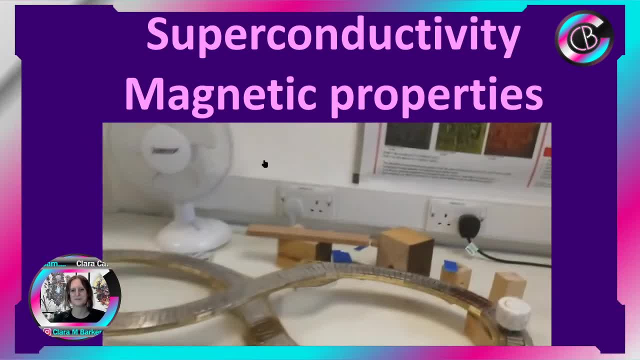 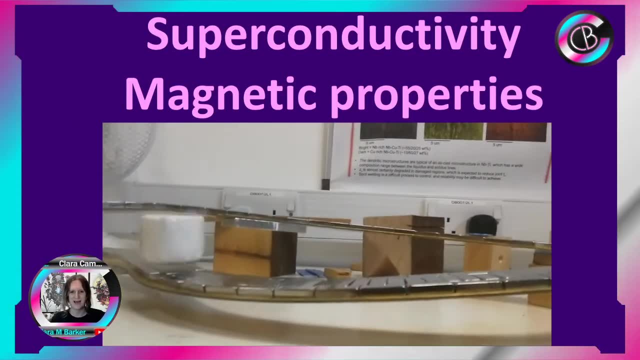 So this is one of my video streams. You can see that I'm going to talk about the properties of superconducting, So this is one of my video streams straight off. so this is a figure of a track of magnets that we glued together in my lab. 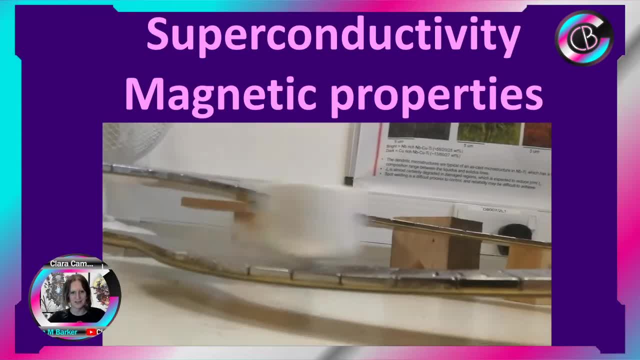 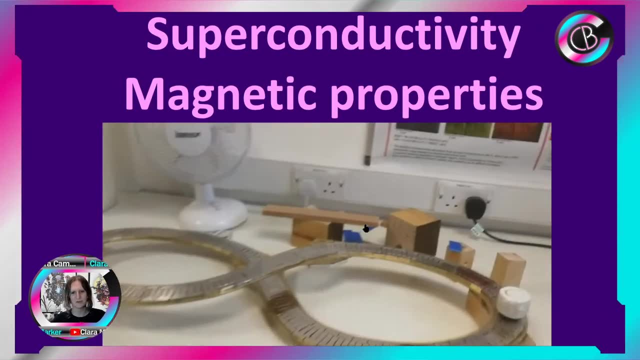 whole bunch of magnets. there's a one pole on the inside and then the opposite pole on the two outsides, and we have a superconductor in a polystyrene cup which we've cut down. there's a little bit of liquid nitrogen in there to keep it cold, because we already know that we've got to. 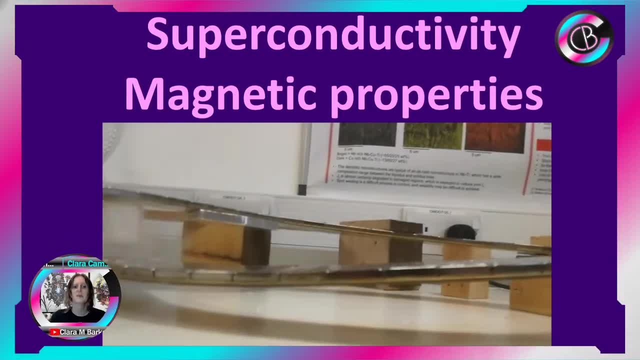 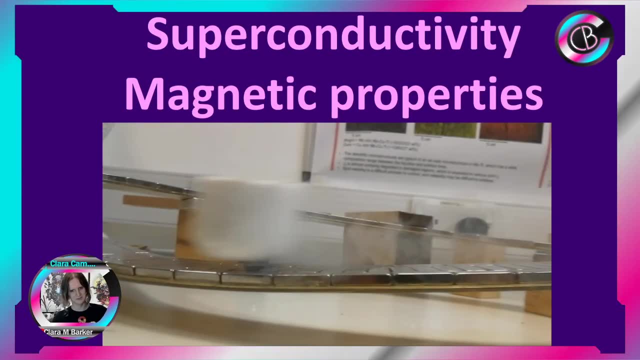 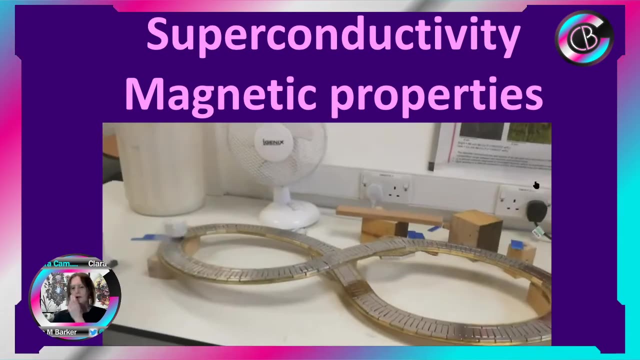 keep it cold, to have our superconducting magnetic properties as well as our electrical properties. it's the same for both, and you might have seen videos like this, where you've got your superconductor floating above or below a magnetic track, so oh yeah, we don't need to watch it again. 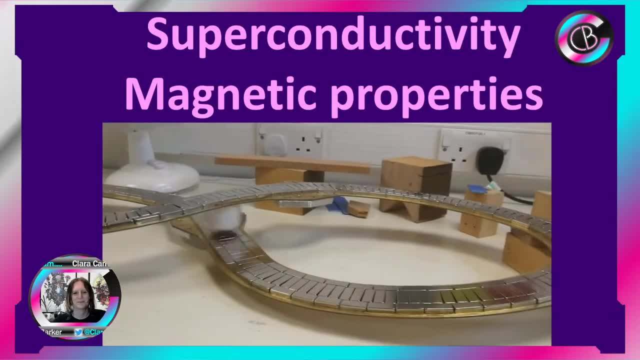 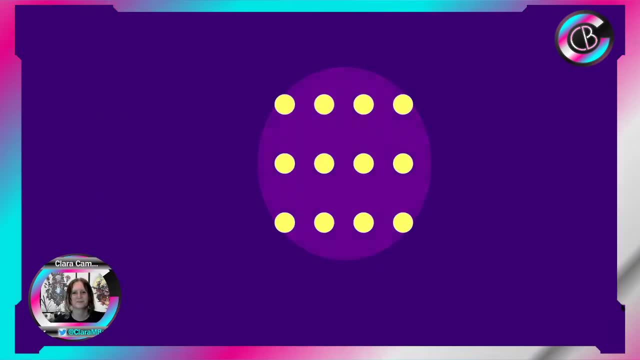 although i know it's kind of cool, right, um, i gotta admit it was fun building this because then we could play around with it. it's not perfect, but uh, yeah, i love it so much fun. all right, so let's take our um superconductor. so, uh, this time, once again, i've- i've put up these yellow balls which i'm 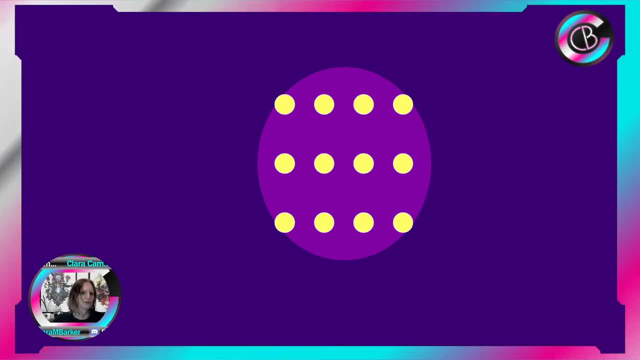 going to say are the atoms of our superconductor. i've not talked about what the material of the superconductor is, and that's not really important for this explanation, but what we have here is a classic superconductor, and so it's made up of all these atoms in a different, particular structure. 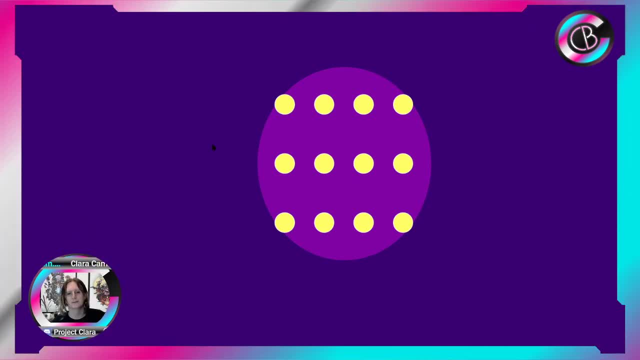 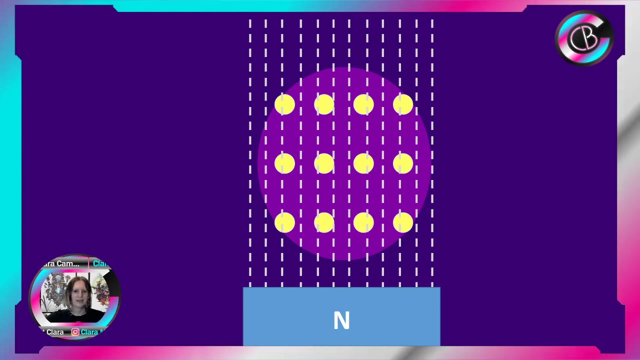 and you know, you've got the bulk, the purple things to signify the bulk, and then the yellow bits of the atoms, right, and then what we do is we introduce a magnet, and a magnet has a magnetic field. so it's not actually, um, you know, a straight dotted line as i've got in the video, but 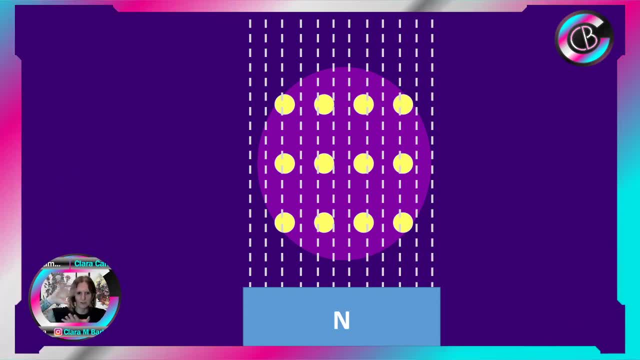 that's just a representation of the magnetic field. so i think we know that the magnetic field will go from north to south and they'll um, and they'll be all different shapes depending on the size and the strength of the magnet. i've just represented them here as straight lines, just for simplicity. 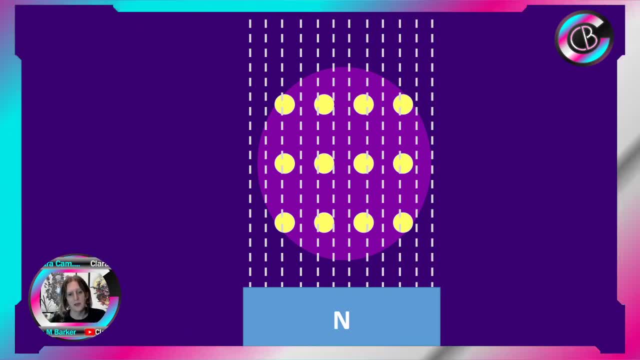 and so if we introduce our permanent magnet and you know, we bring it close to our superconductor, the, the magnetic field lines, the magnetic field will just pass through the material. that's what we expect. now i'm not going to go into the properties of uh. 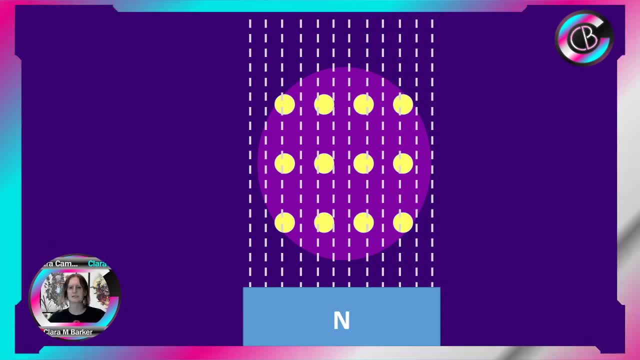 magnetism, but i think we know that some materials will become magnetized and some won't. this isn't what's happening with our superconductors at the moment. the field is just passing through the material. it's not becoming magnetic, it's just passing through it. 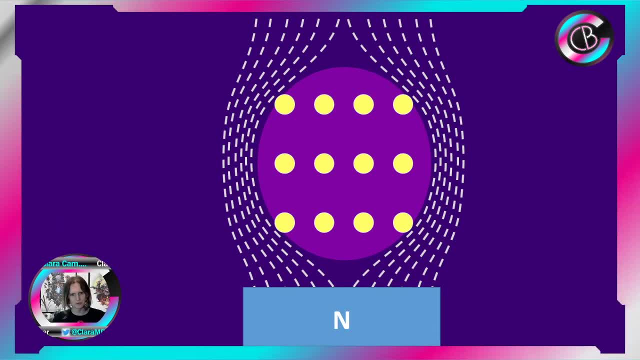 but then when we cool down our superconductor to the critical temperature, then what we find with superconductors is at the same point where all of a sudden they have zero electrical resistance, all of a sudden they expel the magnetic fields. so they basically, if you have a superconductor and 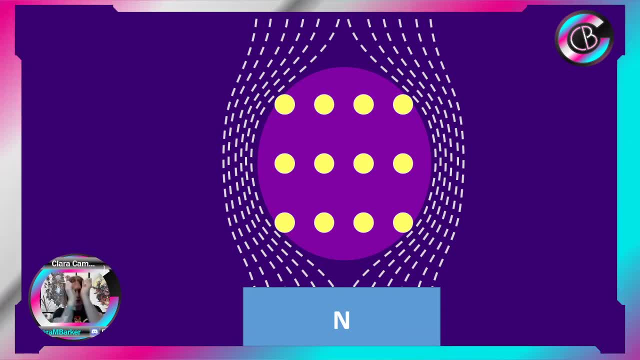 you cool it down and there's a magnet, a permanent magnet, in it, by the magnets, the magnetic field, it's kicked out of the superconductor. it cannot pass through the bulk material and this is really, you know, quite unusual. so if you imagine that you had a permanent magnet and 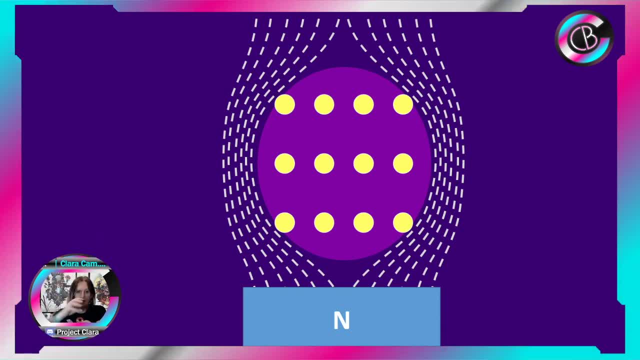 you dropped a cooled superconductor um on it, it would sort of levitate, because there's this force where the magnetic field lines are bending out the way, and so it's. it's not a repulsion per se, it's just it can't move through um, and this is what happens with classic uh superconductors, uh, which 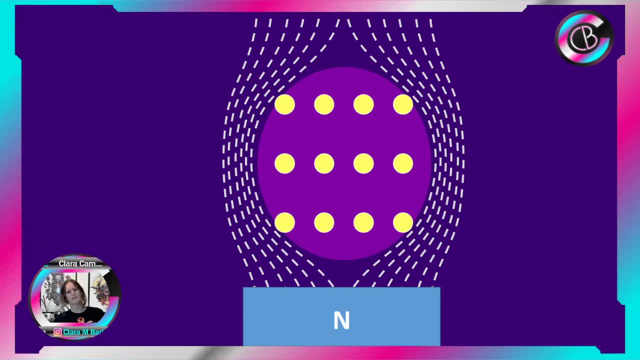 we call type one superconductors. so in the last uh talk about, talk, uh about superconductors and i talked about um superconductors and high temperature superconductors. so that's um, you know, depending on the temperature at which they their superconducting properties, turn on. but within that, 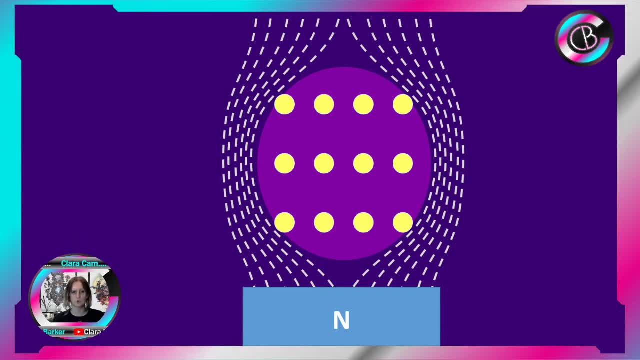 you've also got type one and type two superconductors. so with type one superconductors, when they're cold magnetic field lines, basically they're pushed out, they're expelled from the bulk and they can't travel, they can't pass through it. now, if we take a type two superconductor, 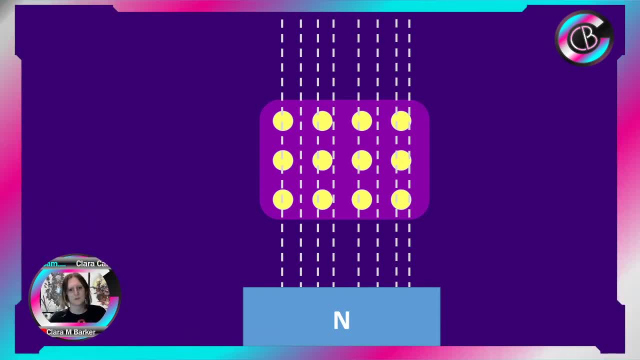 whilst they are warm, so they're above their critical temperature again. the magnetic field just passes through the system like nothing's up. but what happens this time when we cool it down, is that the magnetic fields can pass through the superconductor, but they're pinned. they're. 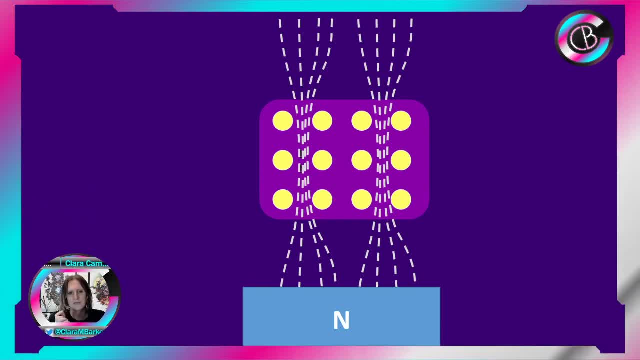 squeezed, they're pushed, they can only go through the material in certain points. so you've got these um these points where the uh flux is pinned, and so that might be um cracks in the grain, it might be imperfections in the structure, it might be um a dopant or something like that. basically, there's certain points within the material that 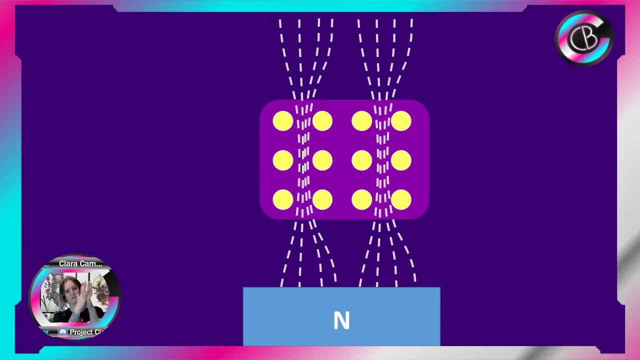 the magnetic field can pass through and so it gets trapped, it gets locked in place and it stays where it is. again, it's not becoming magnetic, but it's just interacting with the magnetic field lines and it's it's locking them in a particular place within the bulk. so with the type one it was on. 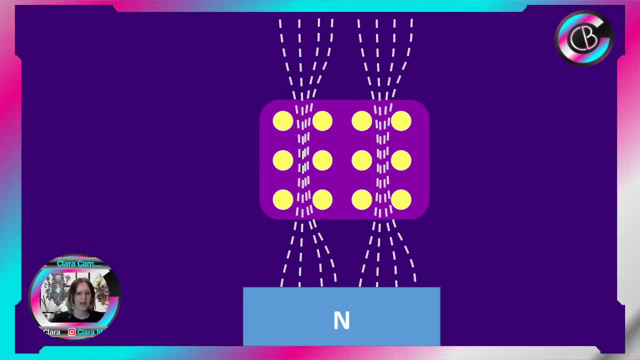 the outside and with the type two it's on the inside. now i should point out that if you cool down a superconductor type two and there's no magnetic field in place, then it'll trap no magnetic field, which on which means that the magnetic field will be locked in place. 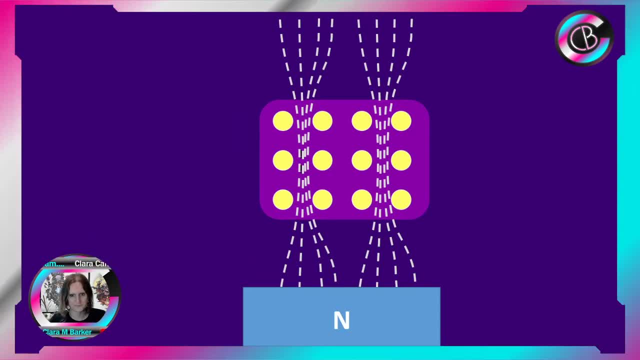 which means no magnetic field can pass through it. it doesn't become type one, it is different, but magnetic fields can't pass through. but if you cool it down in the presence of a magnet, which is what i sort of did here, this is as we're cooling it down, cooling it down, cooling it down in the 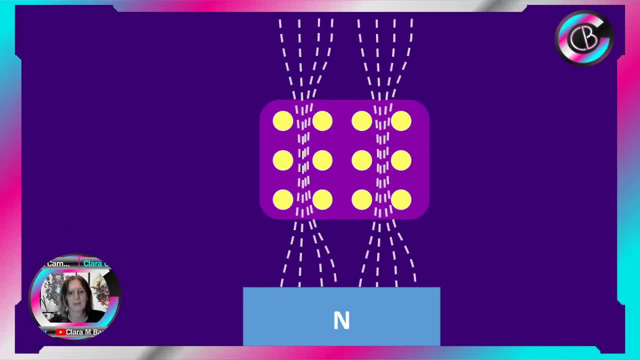 presence of a magnet and, all of a sudden, critical temperature, and we've trapped the magnetic field and it's being forced through these particular points. so this is called, you know, uh, this is how we trap magnetic fields. it's called flux pinning, and what's really? 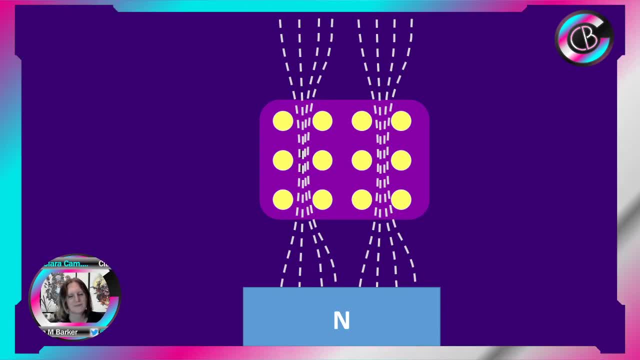 cool is that if you then, having cooled it down, and you keep it cold, if you move the magnet, the superconductor and the magnet want to stay in the same relative position. oh, i'm going backwards here instead of forwards. but so now, if we remove the magnet, what we see is 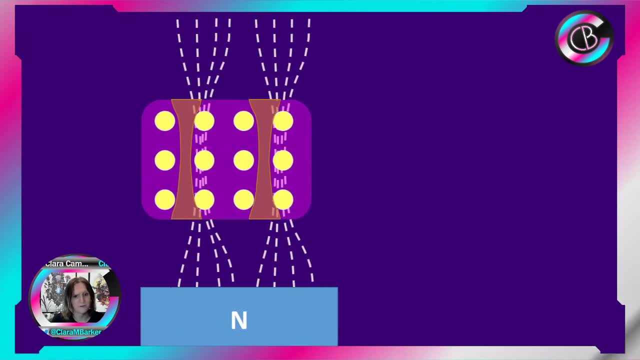 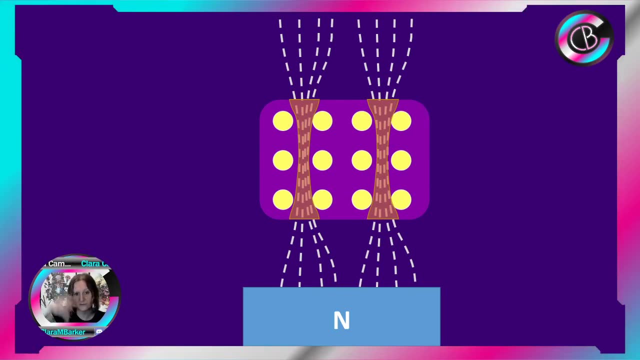 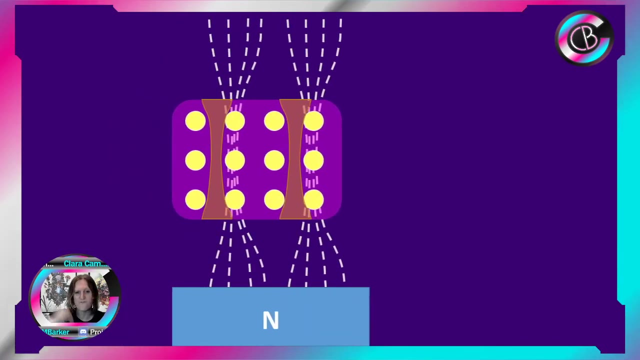 what i'm going to do is just move the magnet and the superconductor goes with it, because it wants to snap to that position. it doesn't want the flux to travel, pass through it in a different position. it'll just move and they'll stay in the same relative position to each other. 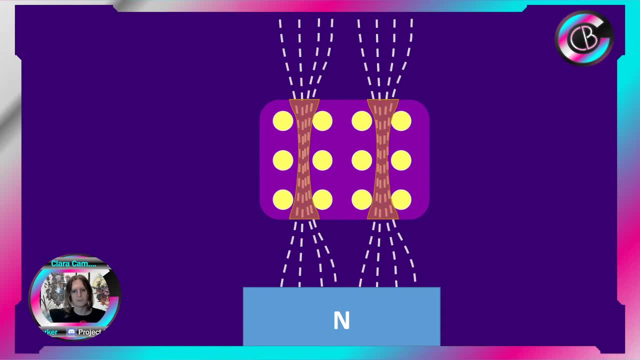 and actually you can overcome that force. you can remove the magnet, uh, and the superconductor, but then when you put them close together, they'll the, the, they'll snap to the same position, the same relative position to each other, and so that's how we get these really cool. 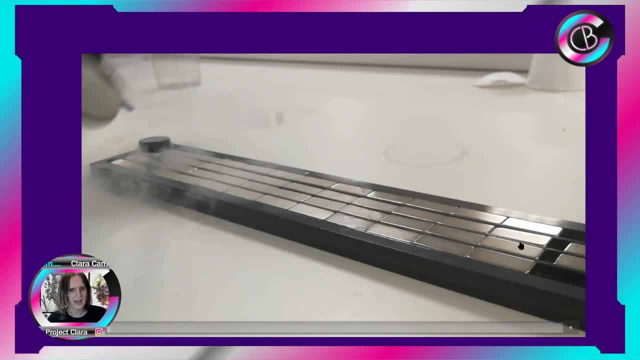 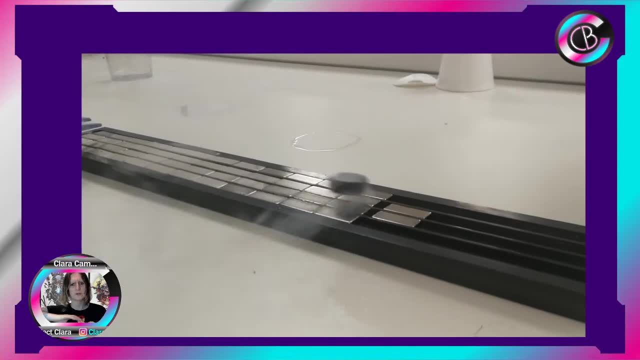 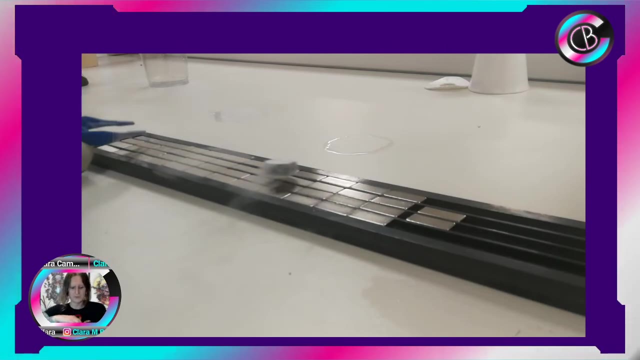 videos. so in the last video I showed this one. this is the basic track with the magnetic field and the superconductor is able to pass along it and it's able to travel along it because the magnetic field is the same. looking at the screen, we're moving the superconductor and in the same direction. 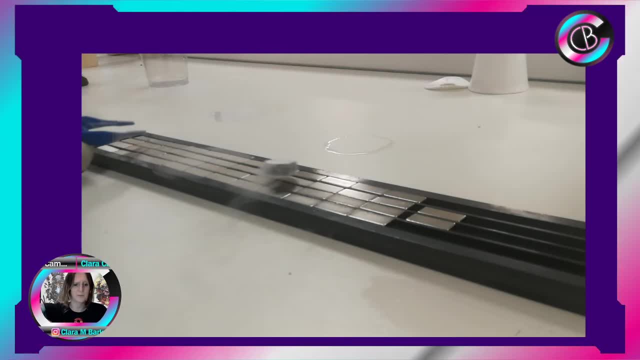 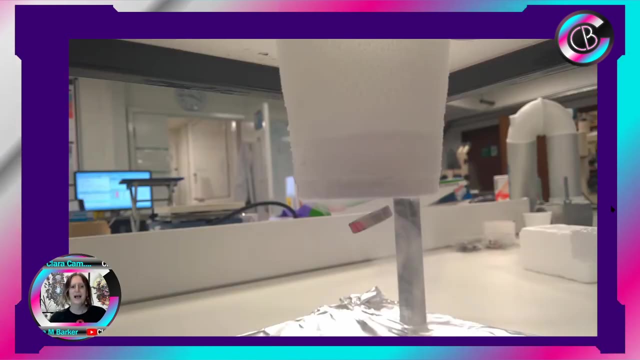 as the central pole, and so it's able to move up and down that central pole because it's the same orientation, but it's not able to travel to the side of it, it's not able to cross the lines of the outer magnets in the track, and so 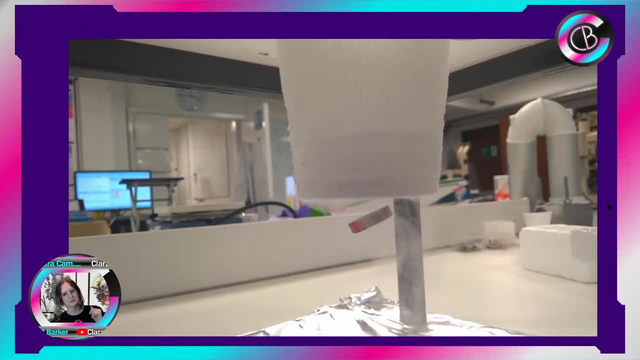 not only can you, you know, float these magnets, their superconductors, above magnets, but you can also do the same in reverse. so here I've actually got a plastic cup with liquid nitrogen and superconductor, and below it I've got a magnet. so I cooled down this superconductor whilst that magnet was in place. and what? 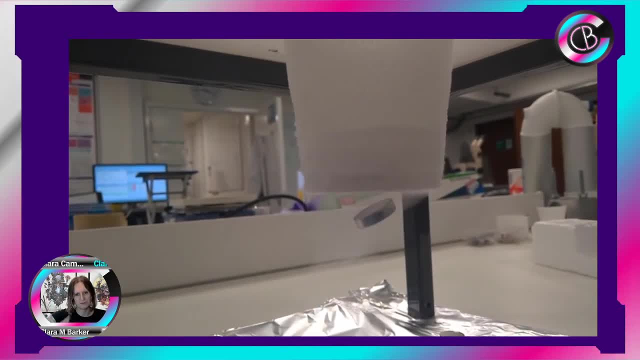 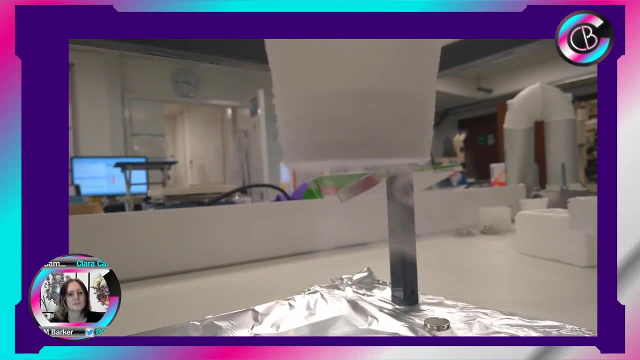 we see is that once I, once it's cooled and I lift up the cup, the magnet is trapped in place. but this time it's below. it's not above, so it's nothing to do with it sort of you know falling on it. it's not like a gravity type effect. 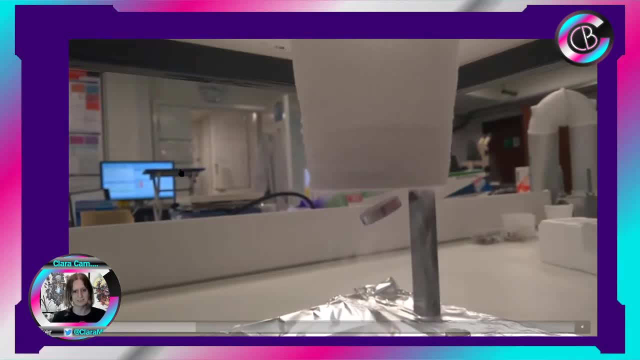 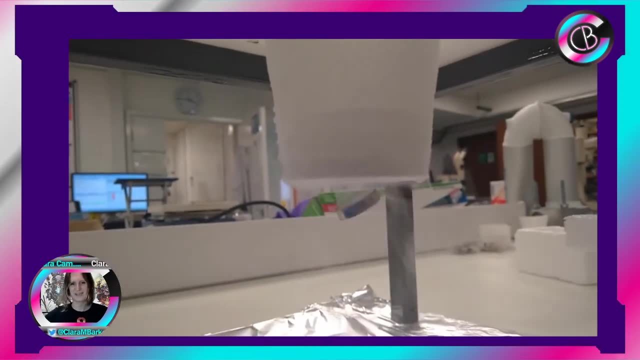 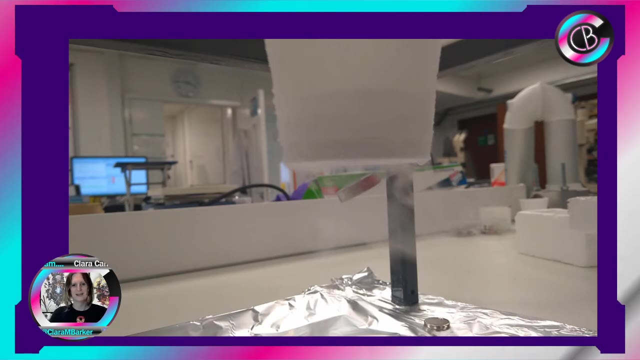 no, it's a relative position. they're locked to each other relatively and you can actually spin. this is a circular magnet, so you can spin it and it's just. it's just really cool and you can get a portion of shaking. it'll stay there. I mean, you can remove it with enough force, but yeah, it'll just stay. 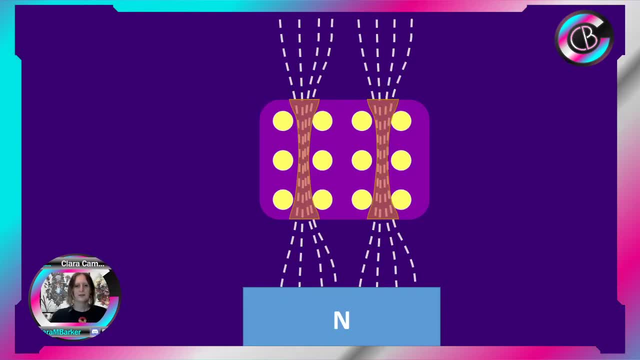 there and you know, in fact we can actually, if you rotate the magnet or the superconductor, then the other will come with it. it's really cool, you can. you can basically go from having a superconductor beforeástico uh uh, you know when you need it and you need it and you can pull it off. it's easily that way. so ween posterior to a magnet isn't? 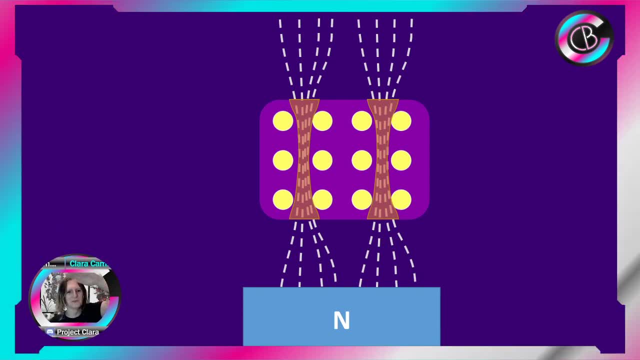 you know, sort of appearing to float above the superconductor, above the magnetic track, to you know suspending below it. And, like I say, it's not that it's suspended or floating, It's just locked relative to each other. 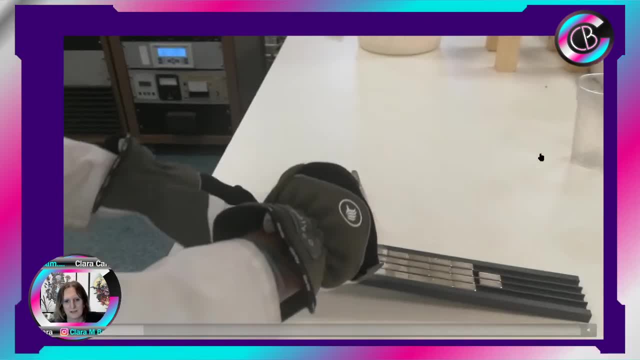 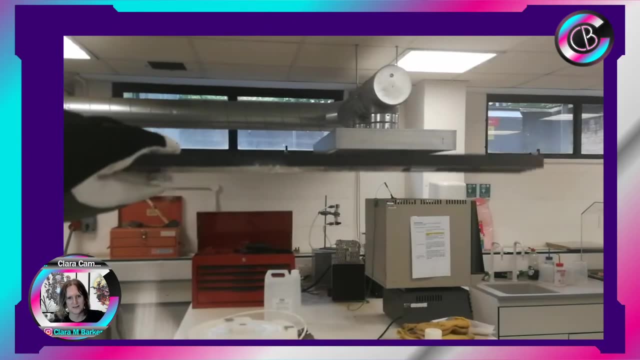 And with a bit of luck it's not the best video, but with a bit of luck I've cooled down the superconductor on my track, And so I cooled down the superconductor and put it on top, while the magnetic track was underneath the superconductor. 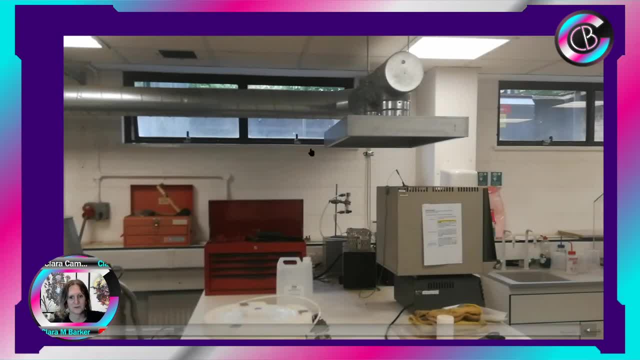 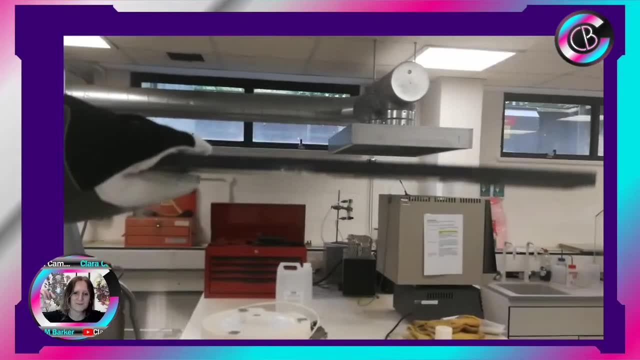 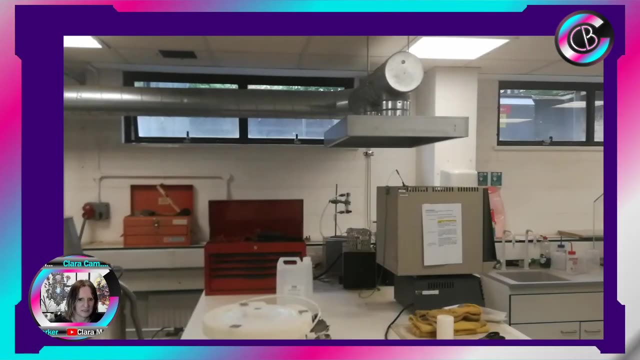 And then I flipped the magnetic field over, turned it upside down and the superconductor stayed the same distance away from the magnetic track, but now underneath. And then, of course, because it'll warm up, because it doesn't stay cold at room temperature, 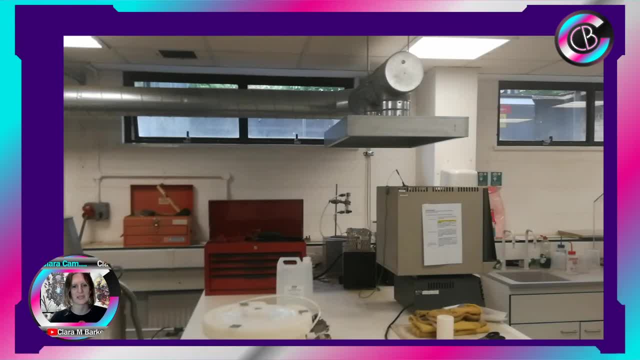 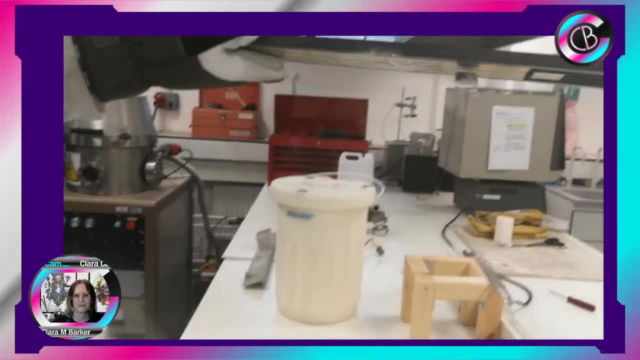 for very long Long without liquid nitrogen, constantly keeping it cold. So it will, you know, suspend. But I think that's really cool. I had loads of fun doing this and just sort of whipping seeing whether we could get it upside down and twist. 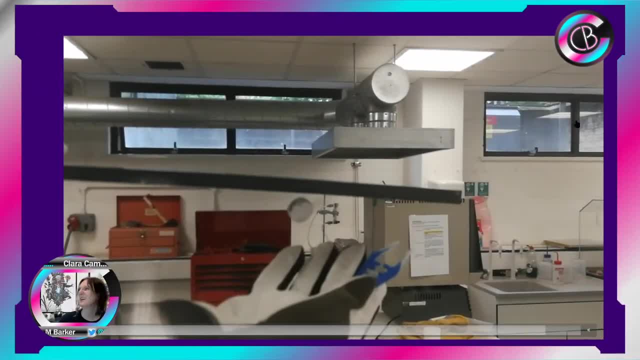 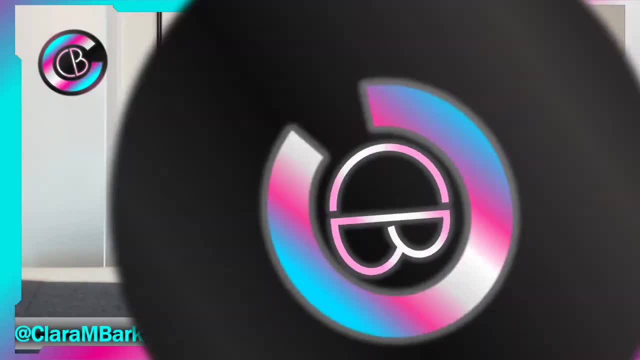 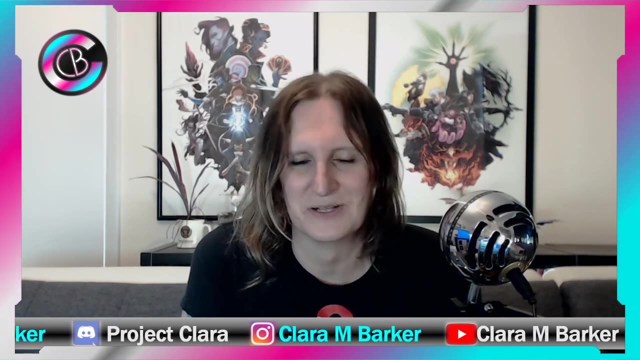 before it warmed up. basically, It's kind of tricky to show really: Yeah, so that's that. So, yeah, so in my last video I talked about the once you reach a certain temperature, you have zero electrical resistance. 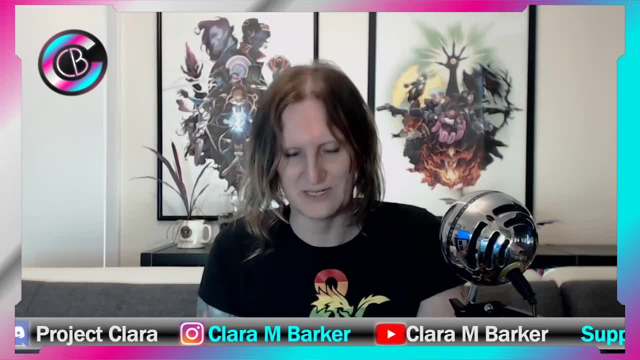 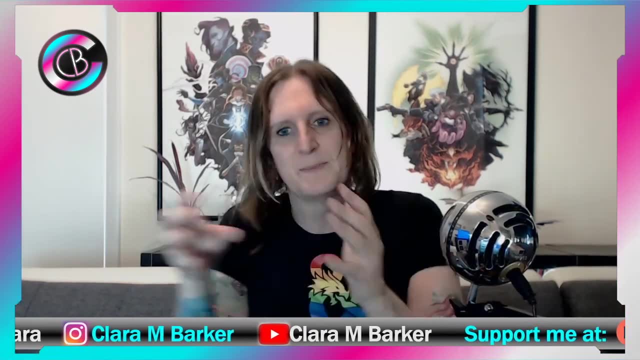 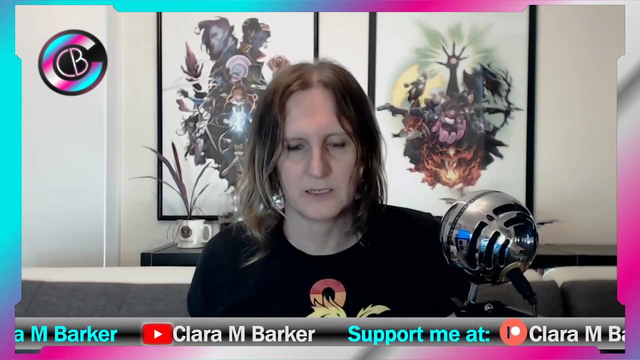 And in this I'm showing the same temperature for the material, So that temperature for the electrical and magnetic properties is the same for a particular material. So if you're talking about, you know, titanium nitride, then the superconducting and electrical properties. 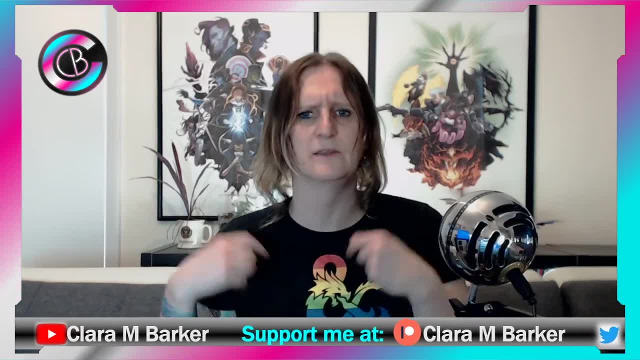 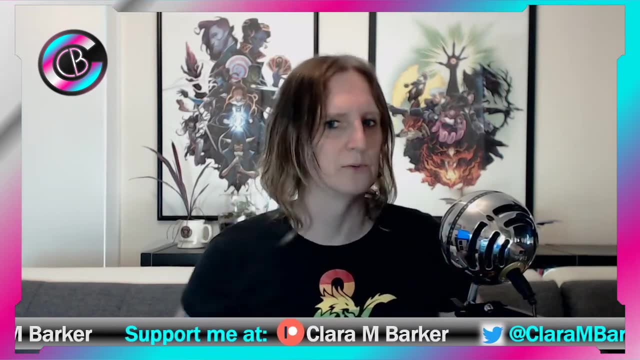 are kicking at the same point. The magnetic and the electrical properties are kicking at the same point, But that'll be a different temperature to materials that we have called Bisco, or, you know, the first superconductor that was observed at Mercury. 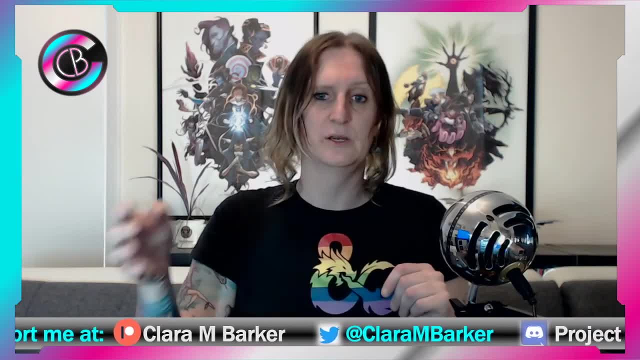 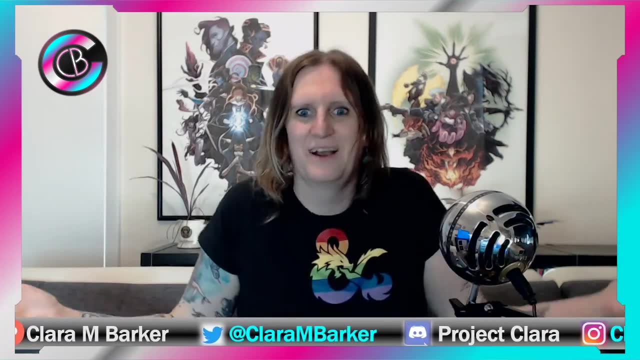 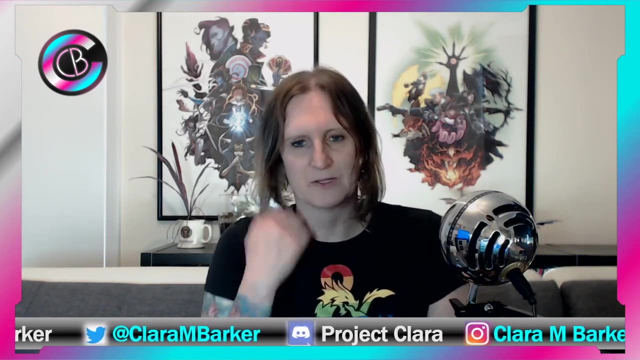 They'll all have different temperatures, but the temperature at which they transition, the electrical and the magnetic properties go at the same time. I think that's pretty cool, But you know, maybe that's just me, So yeah, so that's another video on superconductivity.